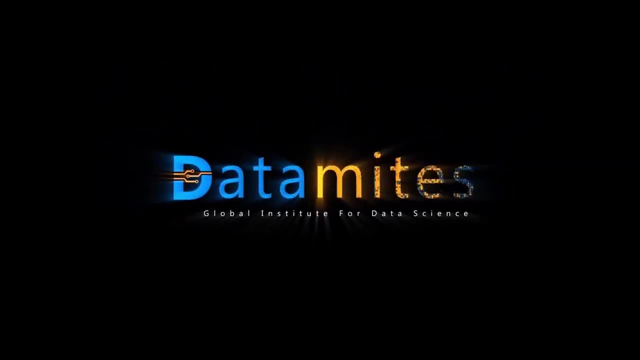 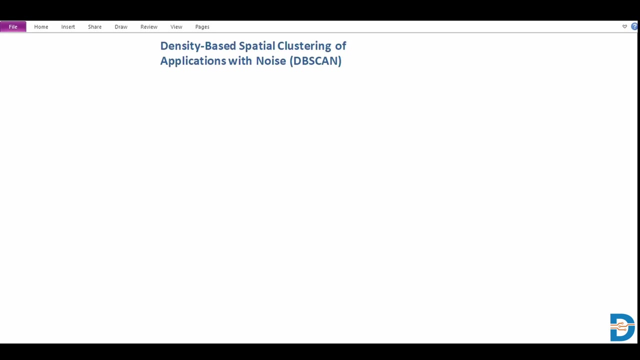 Hello and welcome to this video on machine learning, where we'll be taking a look at a case of unsupervised learning, which is clustering. So we all know how important clustering is, whether it used to be done back in the day, using manual techniques, or we are using the. 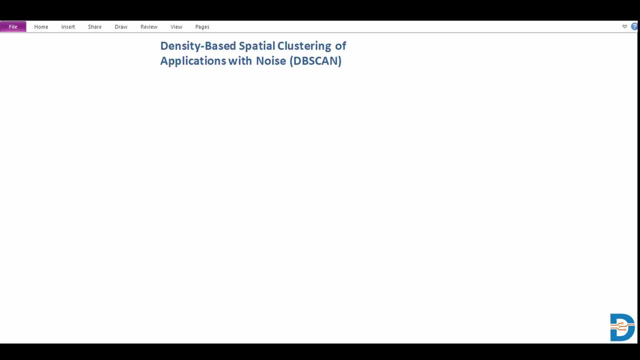 modern day algorithms at our disposal. So db-scan is one of these clustering methods. Essentially, the idea of clustering is to group our objects together based on similarity or based on some similar traits. So, in terms of how db-scan works, let's try and understand. 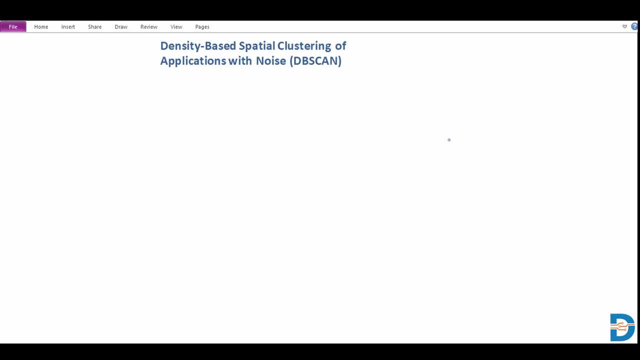 a few essential traits. We have something that's known as a core point. When we talk about a certain observation being called a core point, we are essentially saying that within a given radius, there are a minimum number of samples, defined by a minimum number of samples. Buckle, spreley. Every strength is a constant and may vary based. on the thickness of theistent plate form. And finally, we are called to Shanghai f, but this value based on numberthe rangethe stability, the rangeis joystick-using. if we use the later, We think of this as the use error value balanced between the two elements. This was mentioned before, but you can see there are two zeroes or you get a zeroing 소리. So if we try to make a work, this is as walk through N and that's where the observed data occurs from. And, unlike the linear attitude, we can use the exponents. 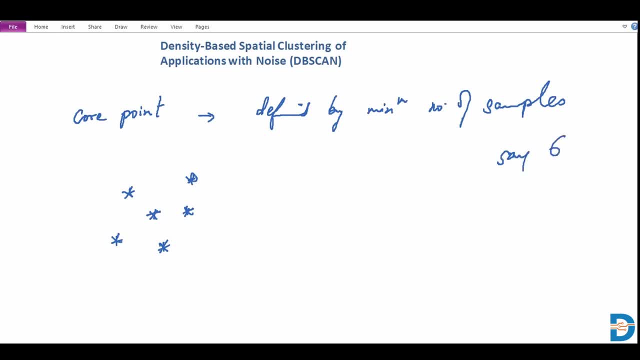 exponents and the coordinates of the agreement, Which is one component that's assigned first to the available six. So a core point becomes a core point if it has at least six samples. we've got five. now let's say another one over here in a given radius around it. that is at least touching about. 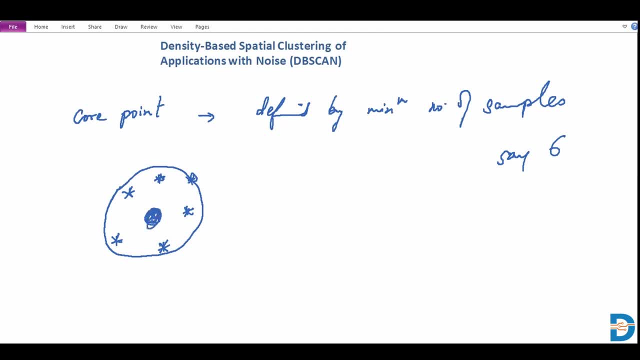 six points, then we can call this particular observation a core point. Now, beginning at some random point here, we will basically take these minimum number of samples. that's one of the parameters for your dbScan model, and the other parameter is what we call. 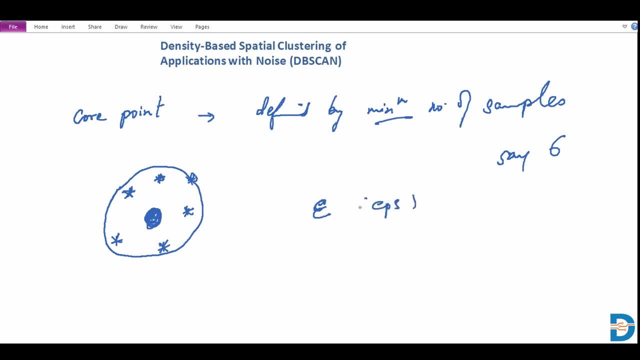 epsilon, or also given by EPS. This is essentially giving us the radius, or it's telling us what kind of the peripheral distance we should be taking in order to say that we need six samples within that radius. So this distance is what we are calling epsilon. So once we have this particular 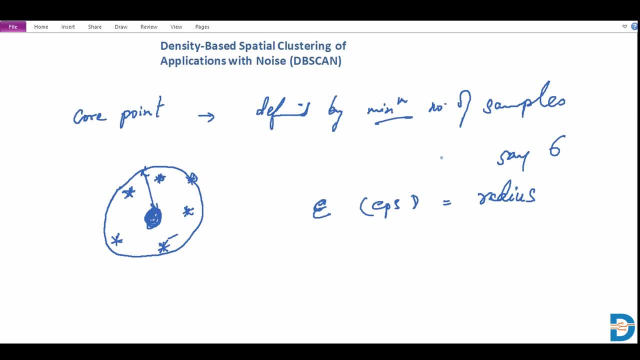 core point defined by the number of samples. as well as this radius, the distance, we can actually begin by creating a cluster and from these points- if this is also a core point- basically we tend to expand our cluster and also include the points that are within the new cluster. 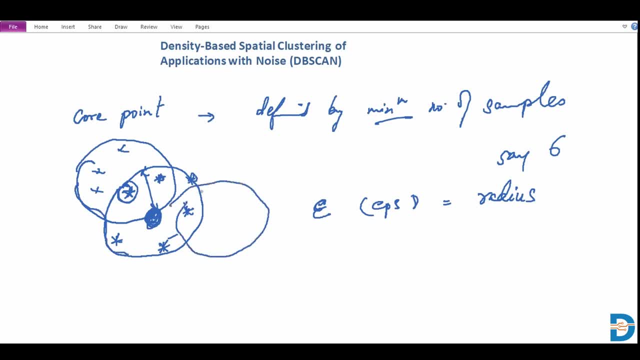 or and in this manner. basically, we are extending our clusters, or rather extending the same cluster that we had started with to create a larger cluster, until eventually we stop at a point where there is a point that doesn't meet the criteria of a core point, which is to say it does not have six observations within that radius of epsilon. 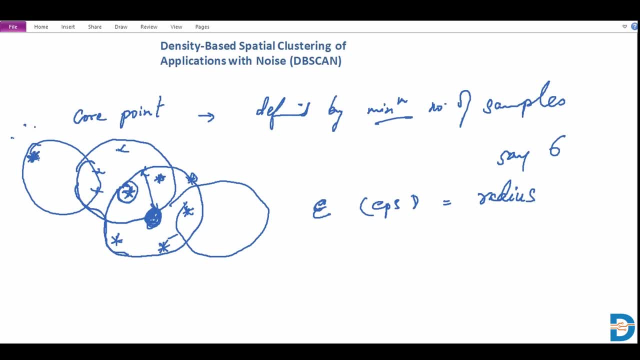 so what we could do is now based on: if this happens to be in that given radius of an existing core point, it gets included in the cluster. it, however, does not allow us to expand anymore. right, we would not be expanding because this itself is not a core point. so that's where we stop. 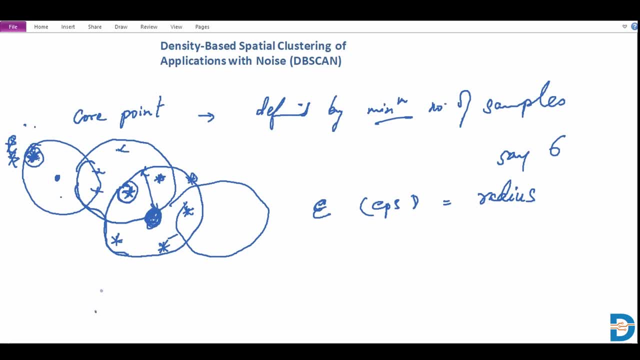 we have created one cluster and we are going to expand it. So that's where we stop: we have created one cluster and we are going to expand it, which may expand in different directions. and then we pick another random point which has not yet been assigned to a cluster and 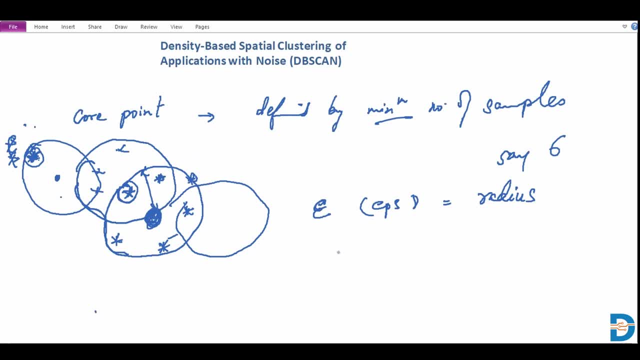 proceed with the same method. eventually, we will have a few clusters with with points that are of a similar density, right we would be. essentially, our clusters are formed based on high density regions and all those points which do not fall in these high density regions, essentially ones that get left out.